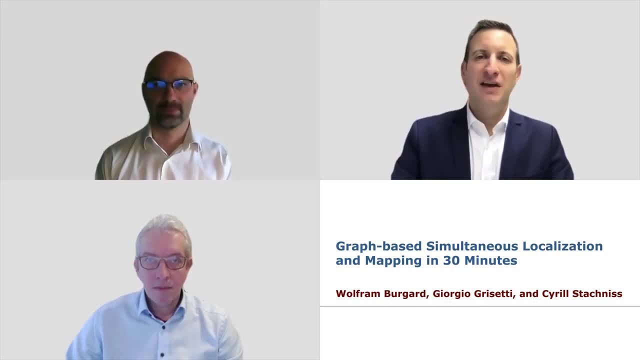 This video lecture consists of three parts. In the first part, Wolfram will introduce you to the basics of graph-based SLAM. In the second part, Giorgio will explain you to solve the underlying least square problem. And in the third part, I will explain you on how to deal with errors in your data association. 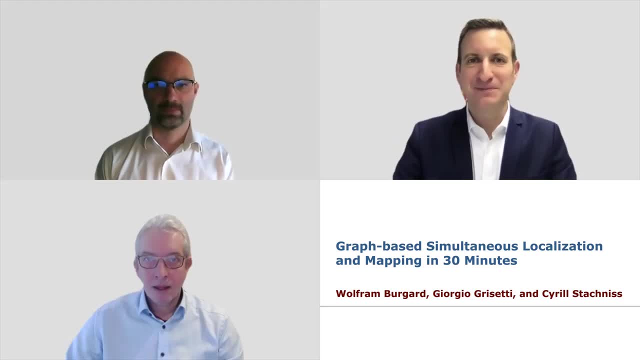 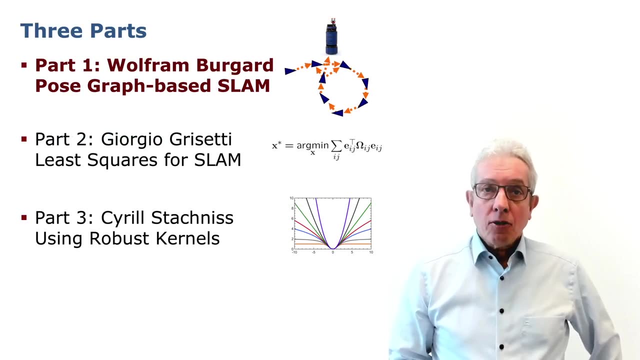 With this I'm handing back to Wolfram. Let's get started. Hello, I'm Wolfram Burgert and I'm going to talk today about the first part of this tutorial on post-graph-based SLAM, taught together with Giorgio Grisetti and Cyril Stadmes. 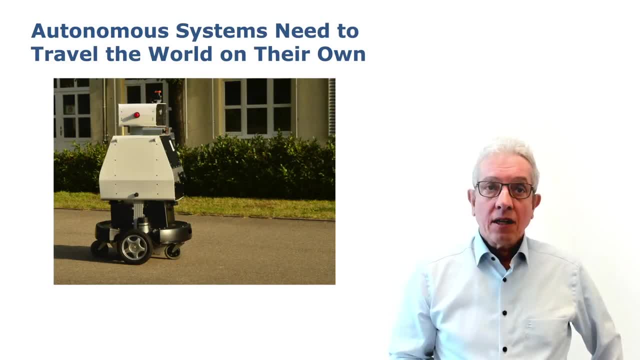 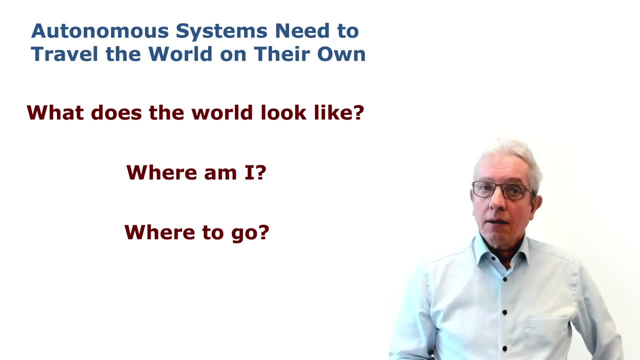 To build robots that can autonomously navigate maps and navigate through their environment, we need to answer a couple of questions, The first one being: what does the world look like? The second one: where am I in this environment? And the third one: where should I go? 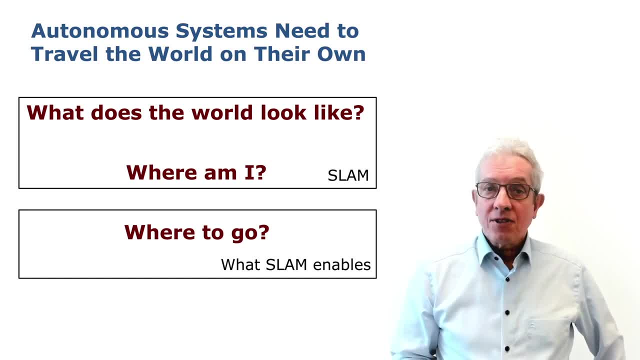 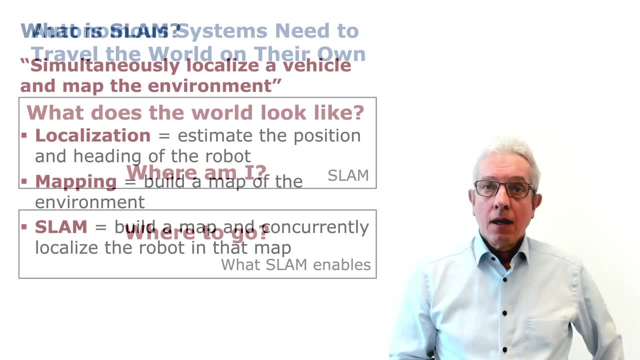 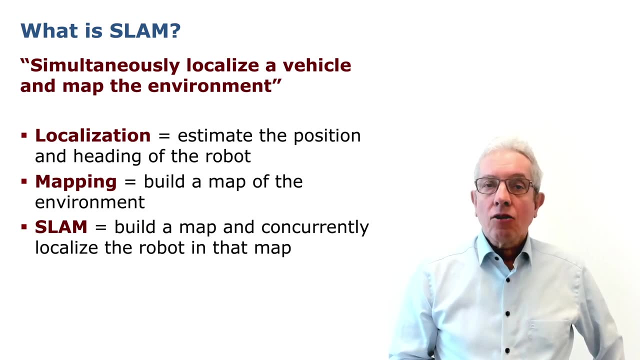 The first two questions are answered by modern SLAM systems, while the third questions are enabled by solutions to the SLAM problem. SLAM is called simultaneous localization. Here localization means estimating the position and the heading or the pose of the robot. 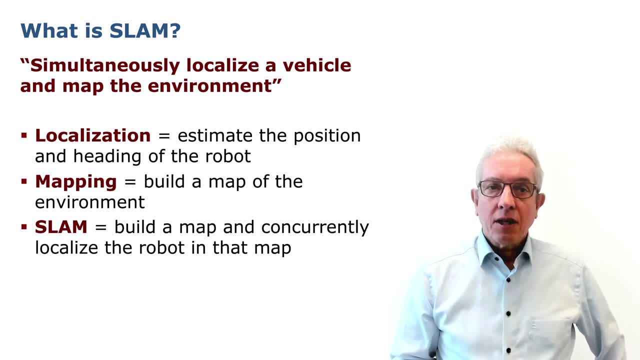 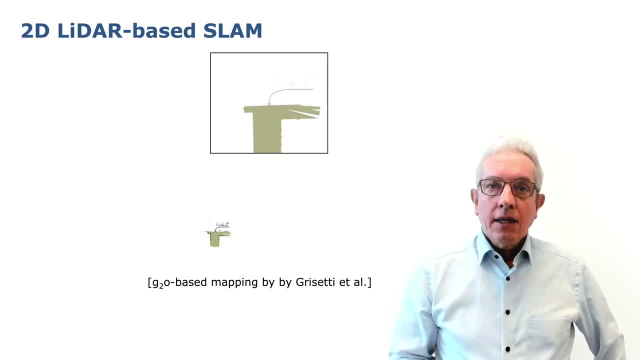 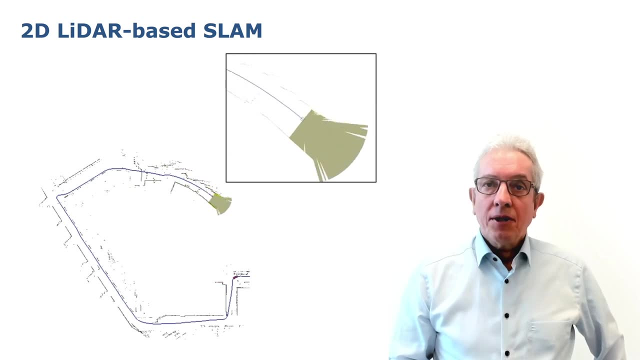 Mapping means building a map of the environment, And in SLAM we need to do both at the very same time. Here you see an example of a robot navigating through its environment and building a map of the environment Whenever the robot comes back to a position. 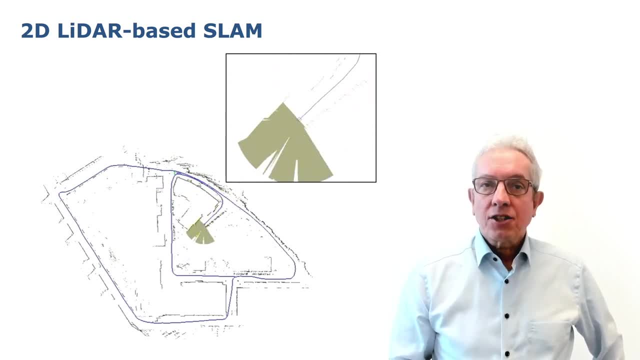 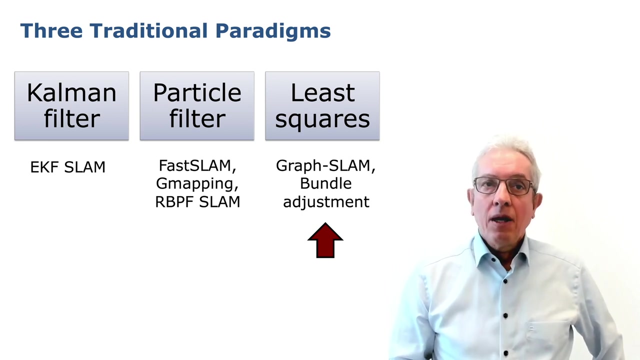 to a place it has been to before. we see that there are corrections made to its trajectory and the map. This is basically what a SLAM process does. There are three traditional paradigms for SLAM, The first one being the Kalman filter type of approaches. 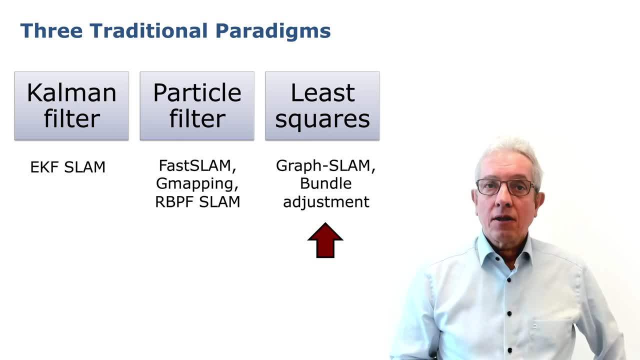 with the extended Kalman filter being the most predominant solution. The second one are approaches based on particle filters or Monte Carlo localization, which are fast, SLAM, G-mapping and Rao-blacklized particle filters. The third approach are the so-called least squares methods. 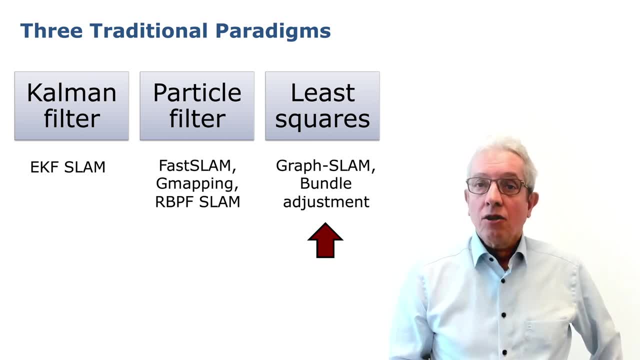 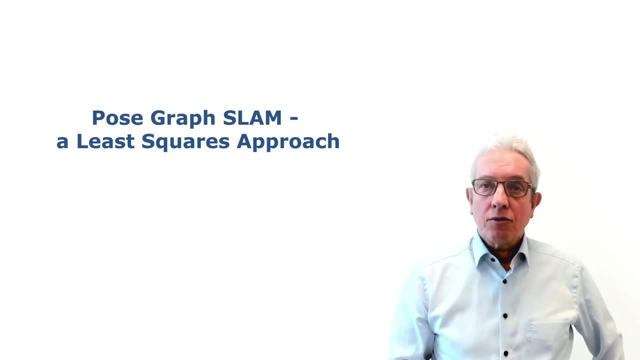 methods with graph SLAM as a predominant solution or bundle adjustment. Here in this tutorial, we're going to talk about the graph SLAM type of solutions. So what is graph SLAM? It is basically the least squares approach to solving the SLAM problem. 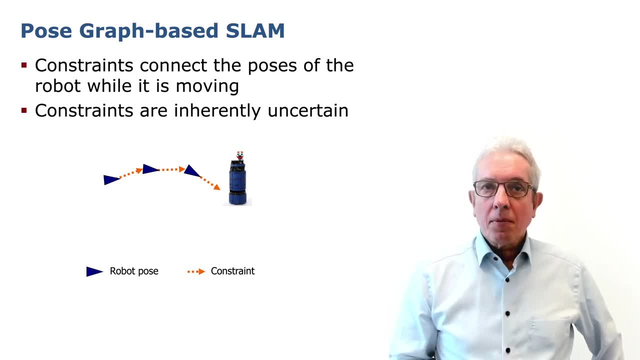 In order to do this, we have to formulate the overall problem as a postgraph, And in this postgraph, as in every graph, we have nodes and edges. Whenever the robot moves, we basically create nodes of the individual positions recorded at discrete points in time. 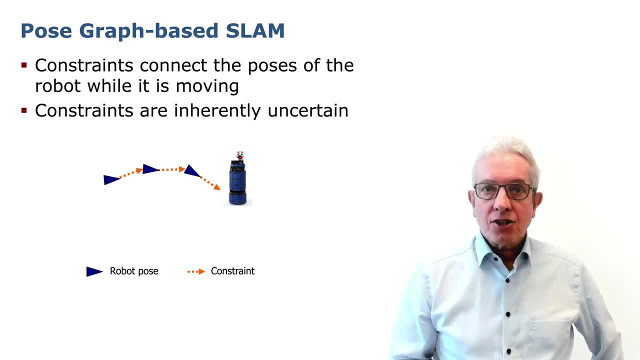 The movements between these nodes correspond to edges that are so-called constraints between the nodes. They basically tell us what the relative pose of these two nodes should be. Obviously, because these are measurements, they are inherently uncertain Whenever the robot gets back to a place it has been to before. 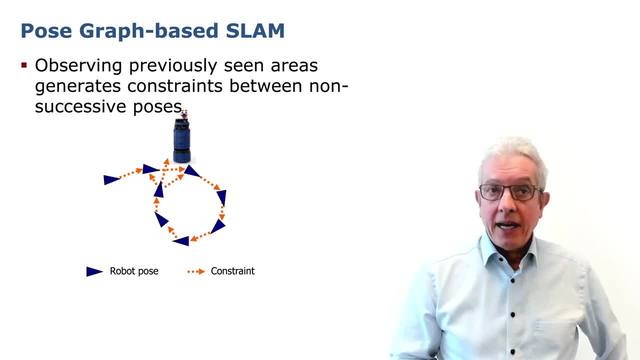 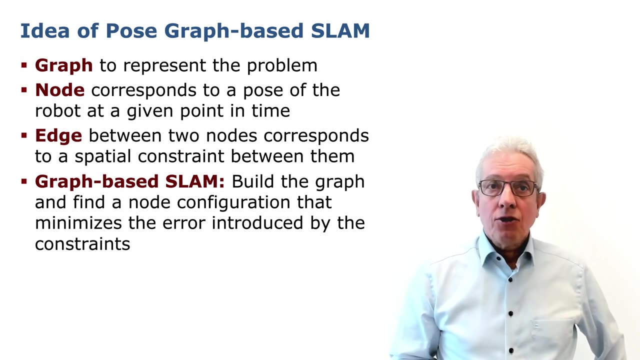 and observes this with its extra-receptive sensor, a LIDAR or a camera- then we generate additional edges or constraints between the corresponding poses. This gives us the so-called postgraph. The overall idea is to use a graph to represent the overall problem. 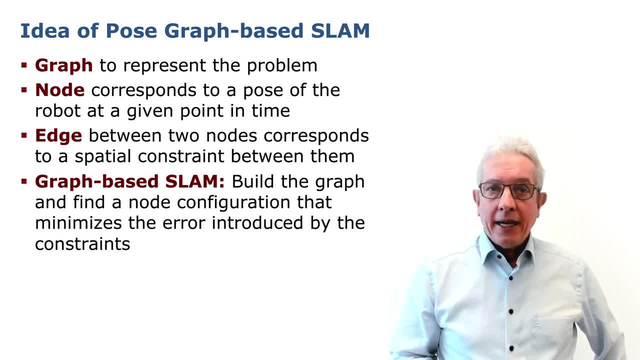 with nodes corresponding to the pose of the robot at a given point in time and an edge between two nodes corresponding to a spatial constraint between the adjacent nodes. Graph-based SLAM basically means building a graph and finding a node configuration that minimizes the error introduced by the constraints. 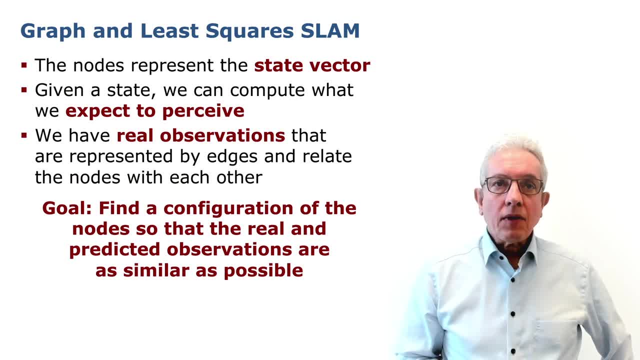 And how is the error formulated? So let's first talk about the state vector, which is basically the collection of all nodes in the graph. Once we have these nodes and the corresponding poses, we can calculate what we expect to perceive. On the other hand, we have real observations. 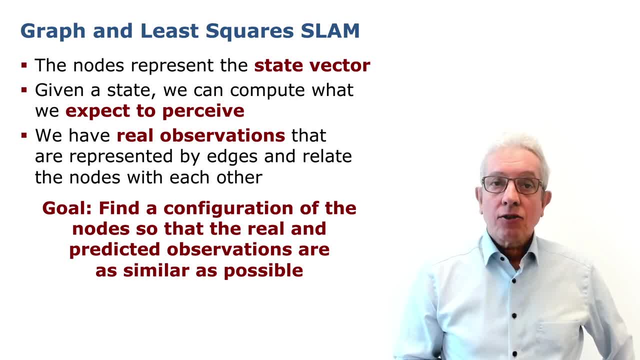 that are represented by the edges and relate the nodes with each other. The goal now is to find the node configuration that minimizes the error between the predicted and the real observations. So, basically, what we are doing is we are taking the state consisting of all the nodes. 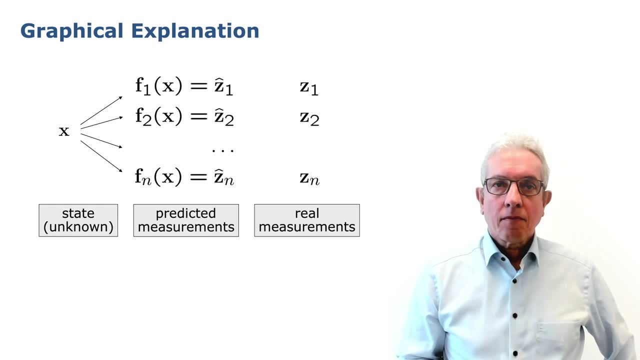 and calculate the predicted measurements for every measurement that we have, And then we compare the every predicted measurement with the real measurement, The error function basically being just the difference between the two. We assume that the measurement error has zero mean and is normally distributed. 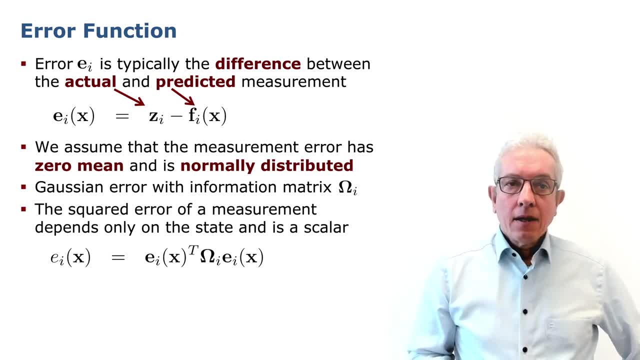 and that we have a Gaussian error with information matrix omega i. The squared error of a measurement is a scalar and depends only on the state. EI of x is basically EI of x. transpose omega i: EI of x. The goal now is to find the state x star. 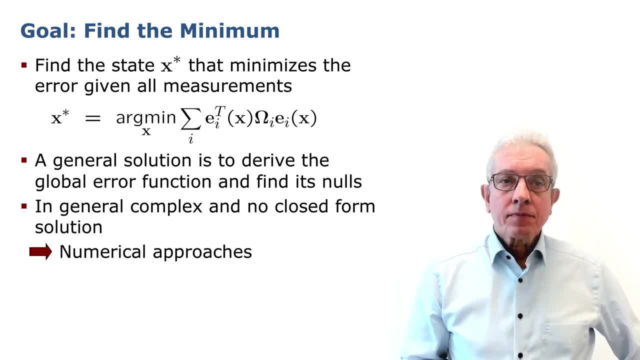 that minimizes the error given all the measurements. A typical solution to solve such an equation is to calculate the derivative of the error function and determine its zeros. Unfortunately, this is, in general, a complex problem for which no closed-form solution exists, which means that we have to rely on numerical approaches. 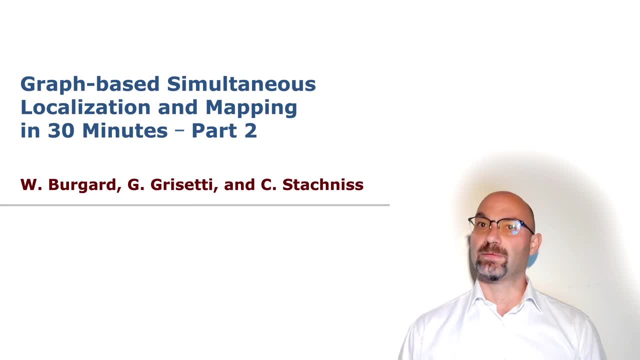 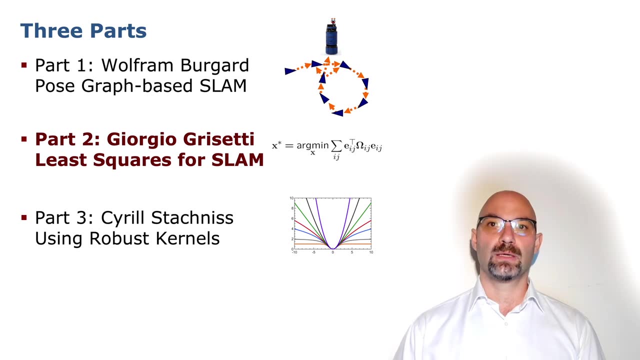 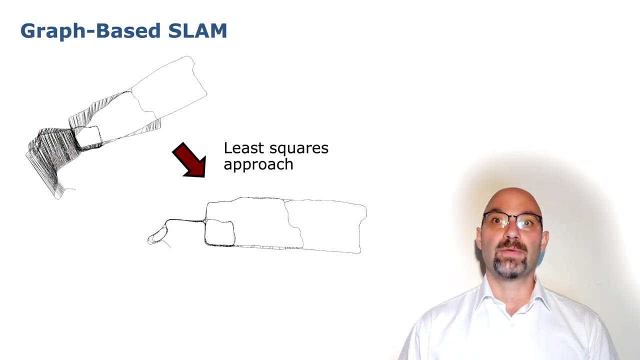 to solve this equation. In the first part, Wolfram was telling you how to represent SLAM as an optimization problem. In the second part, we will investigate about the structure of this problem and how to solve it. We have to remind that, in the end, our ultimate goal 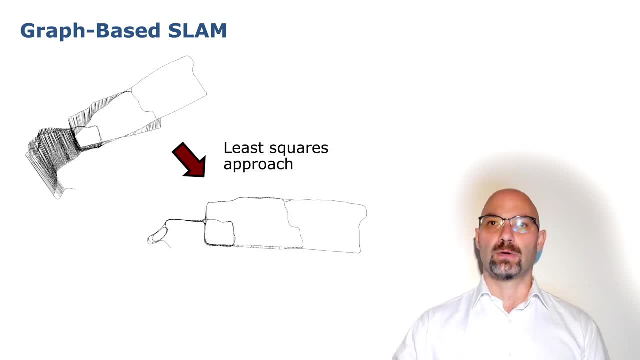 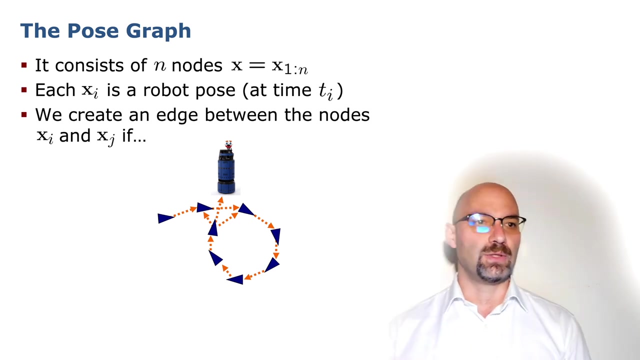 is to calculate the configuration of the robot trajectory that is maximally consistent with the observation. This means that we would like to go from a situation like the one depicted on the top left to the one depicted on the bottom right of this line. The entire minimization problem could be boiled down into a graph. 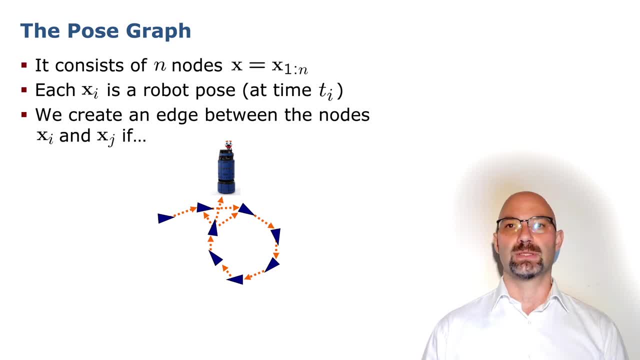 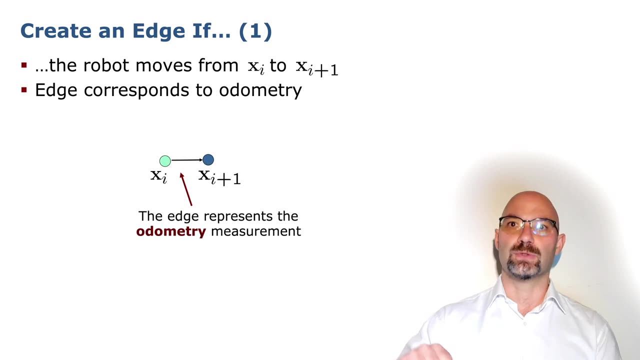 The nodes of this graph represent the robot positions along the trajectory, and the trajectory, in contrast, represents virtual measurements. Such virtual measurements between pairwise nodes might arise either from odometry measurements that directly estimate the radial position between two temporally consequent robot positions, or they can be estimated by registering. 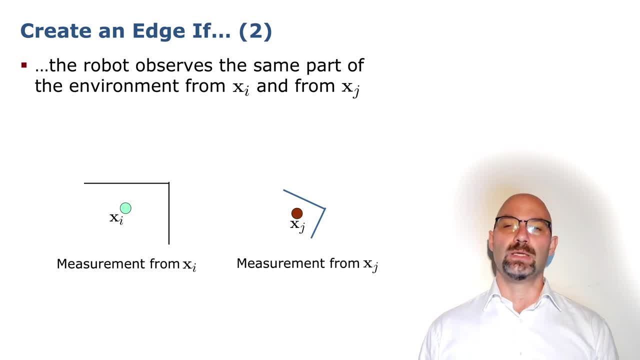 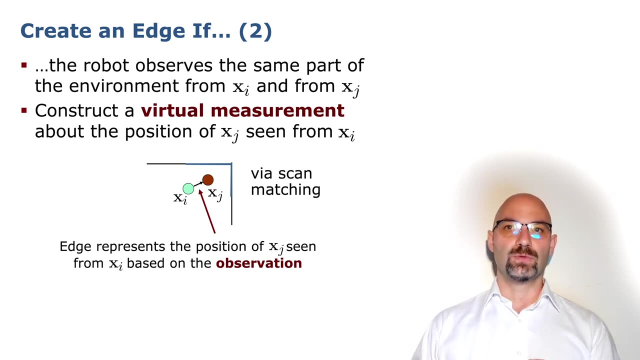 pairwise environmental measurements in order to find their maximum value. We recall that registering environmental measurements, such as scans, would then return a position of the sensor, of the two sensors, that results in the maximum alignment between the two clouds. From this relative position we can then extract a measurement. 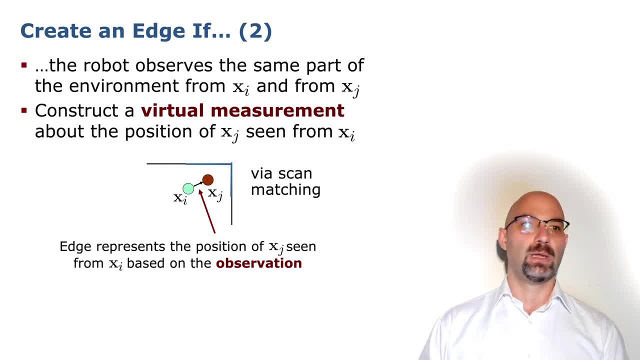 that we feed and we use to construct our optimization problem. Both edges coming from the odometry and edges coming from the registration process have the same type, which is a relative pose, So we can treat them homogeneously. We recall that correctly estimating this virtual measurement. 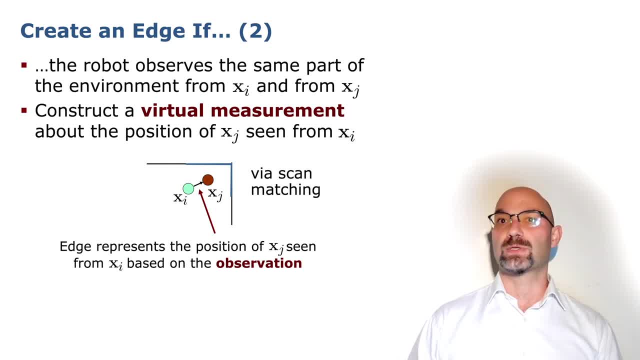 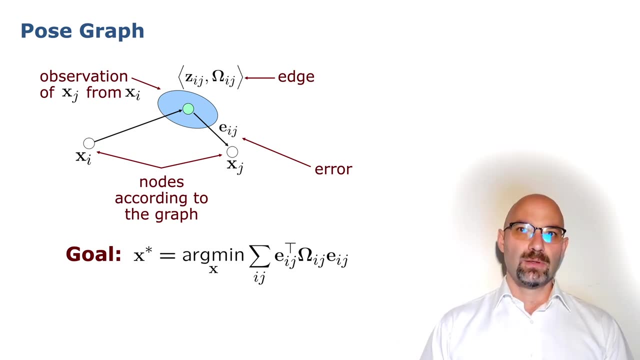 is of crucial importance for an optimization problem, because otherwise what we try to solve has no meaning, and so will be the resulting map at the end, And so it will tell us about it. Now let's look a little bit inside one of these virtual measurements. 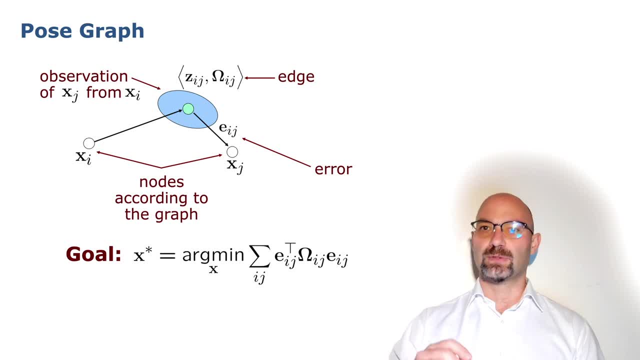 We already said that a virtual measurement encodes a relative position between two dots. This slide illustrates a simplistic two-poses graph optimization problem. The blue dot and the blue circle represent respectively the measurement and its associated uncertainty. We immediately see that we could solve this problem. 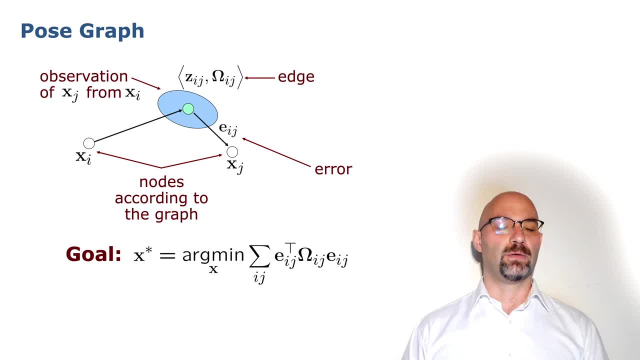 by bringing the node xj in the middle of the blue ellipse of it. Therefore we would be zeroing the error vector. But in general, a SLAM problem contains many variables and many edges that do not agree with each other. However, finding the global configuration x star. 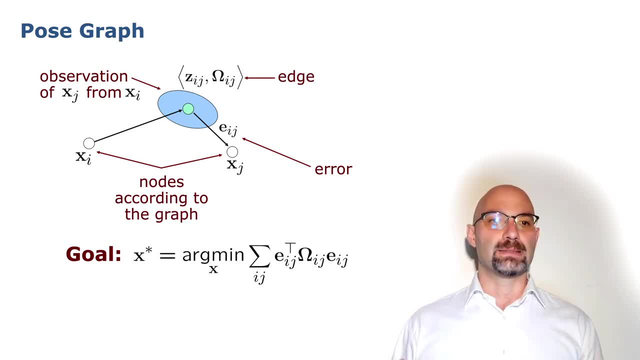 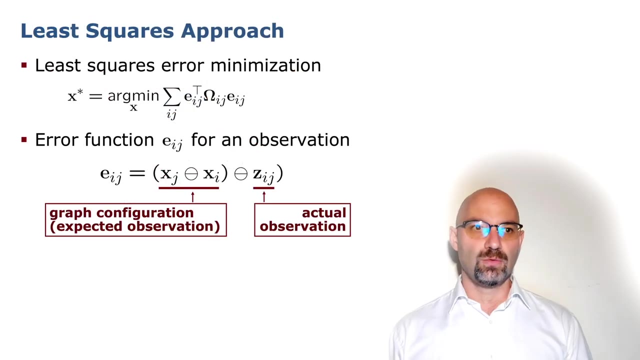 that makes all edges, minimizes the square error norm of all errors, would lead to a potential, potentially the maximally consistent project that exists in terms of the measurement that we put in the problem. Let's now look a little bit inside one of these error functions. 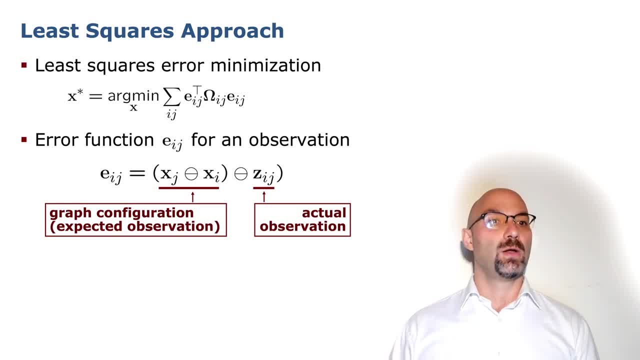 and we can distinguish clearly two aspects: One aspect which is the prediction, which is obtained by calculating the relative displacement between the two poses, And the second aspect is the absolute measurement. We clearly see that whenever the prediction or the relative estimate between the two poses, 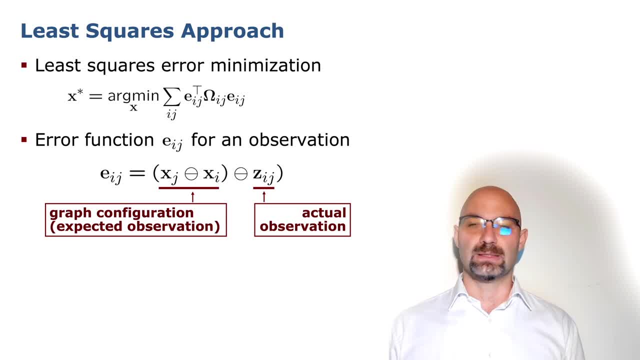 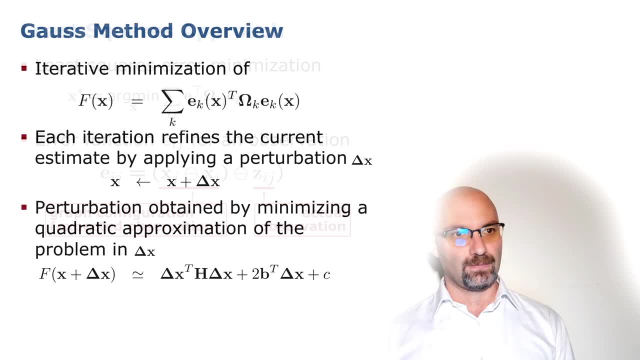 is exactly the same as the measurement, then this error vector is zero. So this tells us that our optimization problem is, at least formally, well-placed. We observe that the shape of the error function of the global cost function that we want to minimize, 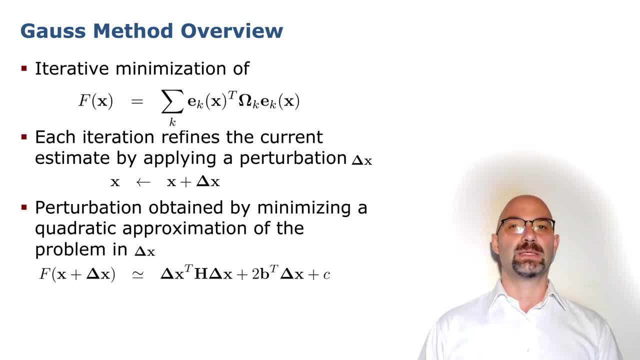 is characterized by many quadratic terms. Such class of problems is well suited to be approached with iterative minimization methods that start from the initial guess of the solution and iteratively refine it by applying the perturbation delta x. Such perturbation is obtained by constructing: 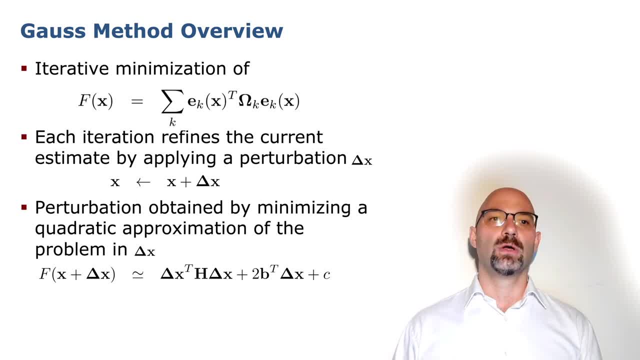 local quadratic approximation of the original problem in the perturbation delta x, And then the perturbation itself is calculated by finding the minimum of these quadratic terms. In this case we have a quadratic form which is the multidimensional extension of a second linear polynomial. 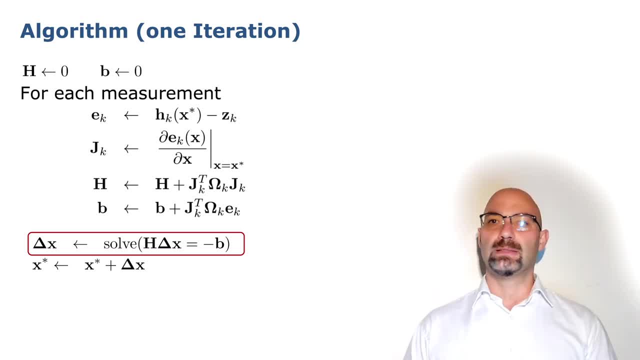 In this slide we summarize one iteration of the minimization algorithm. We can easily see that the goal of one iteration is to construct a quadratic form represented by the H matrix and the B vector, And this is done by linearizing the error function around the current optimum x star. 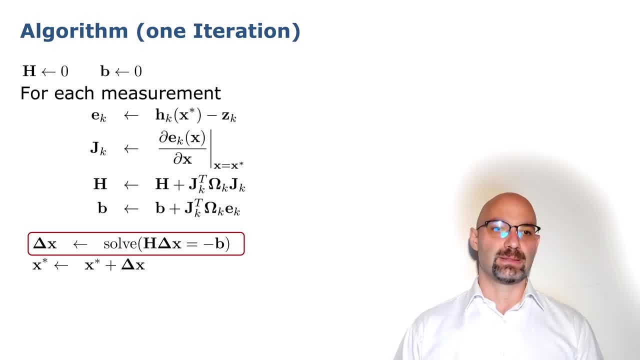 and by assembling the linear system H and B. A crucial aspect in this slide is the solution of the linear system. that can be very large-dimensional. However, the solution of the linear system would lead us to the perturbation delta x. This applied to the current solution. 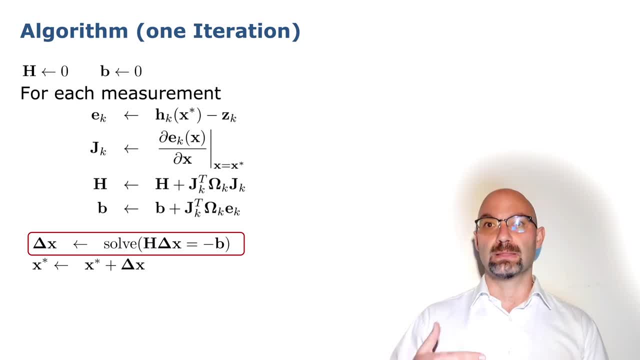 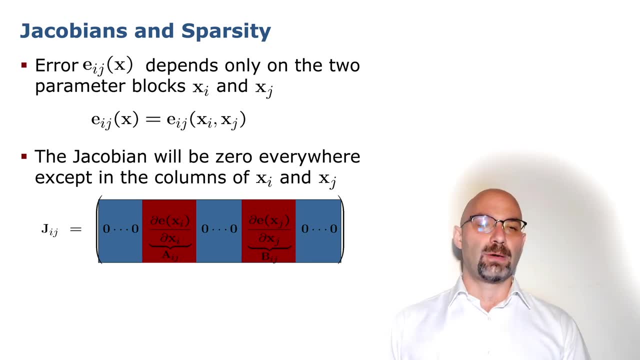 would improve potentially the value of the cost function, which means decreasing it. Luckily, this problem would not be solved if it would be dense, given the size of the problem itself. But luckily the structure of the problem comes to our help because we could observe that the error functions. 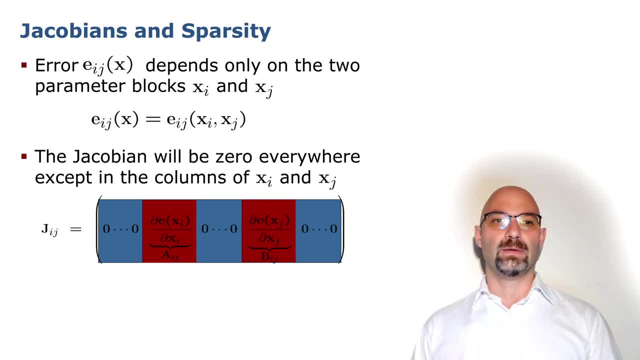 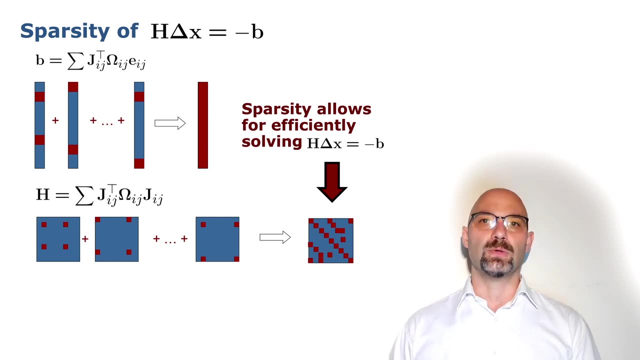 are only affected by the pair: the value of the two variables that they connect. This means that the Jacobian will be non-zero and only in correspondence of the block, And this means that once we construct the quadratic form, each error will contribute only. 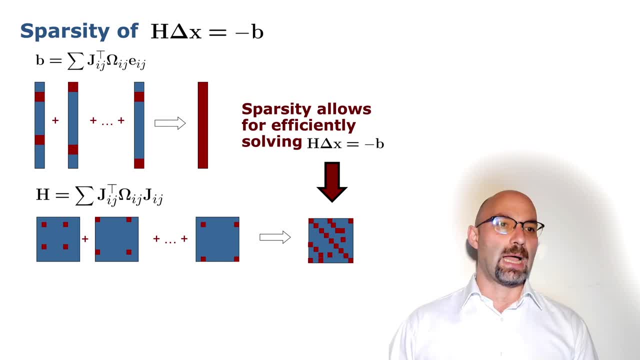 with one single non-diagonal component. Normally we have a number of edges which is proportional to the number of nodes, given the structure of the slump problem, And this will lead to a system which is definitely sparse and can be actually solved with modern linear solvers. 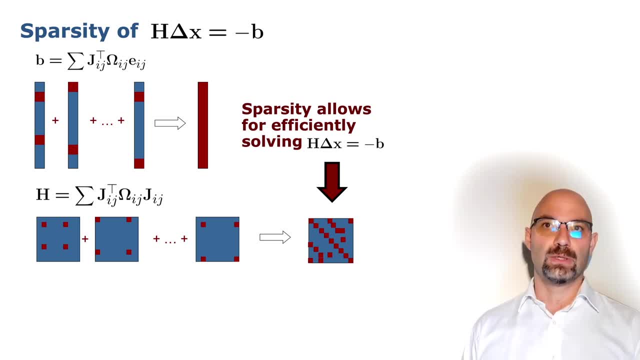 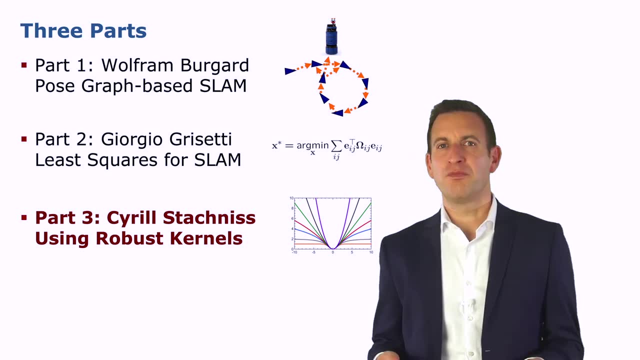 such as C-spars or Cholmonde. And with this I conclude my part and I leave you to see what's next. In the first part, Wolfram introduced the idea of pose graphs and how to use pose graphs for modeling the slump problem. 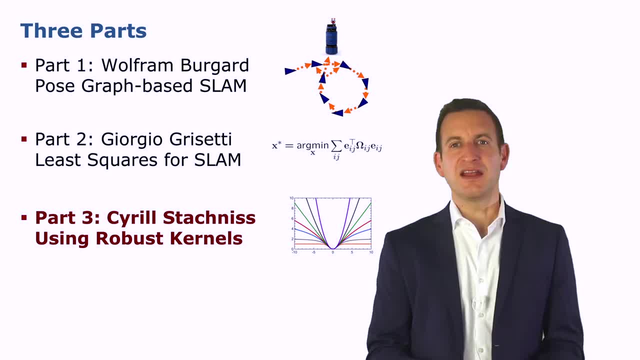 In the second part, Giorgio told you how to use the ideas of these squares in order to minimize the errors introduced by these constraints, And I will talk now about how to use robust kernels in order to be more robust with respect to errors in our data cessation. 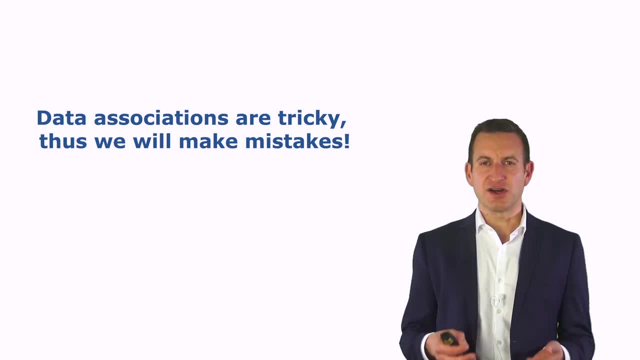 So we start with the observation that data cessations are tricky to do and thus we will make mistakes in the long run. We simply can't prevent that, Though the question is: how can we deal with outliers and gross errors that we are doing when we are building up the SLAM graph? 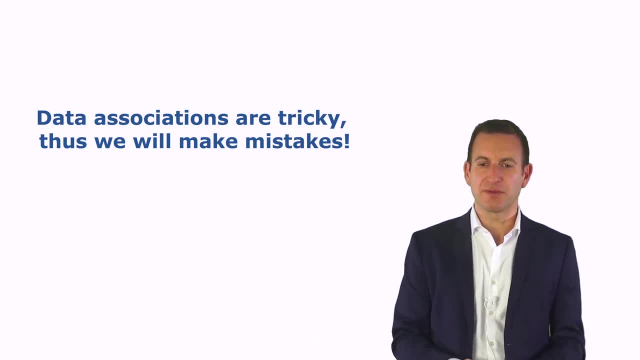 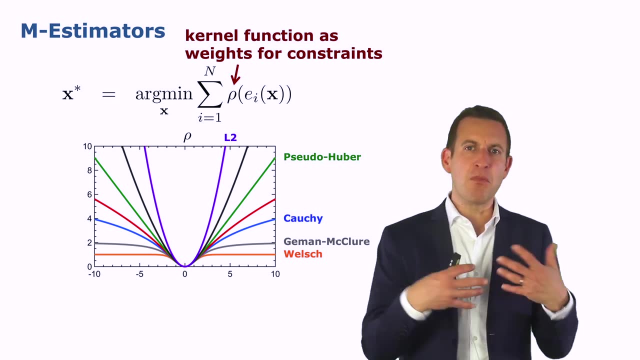 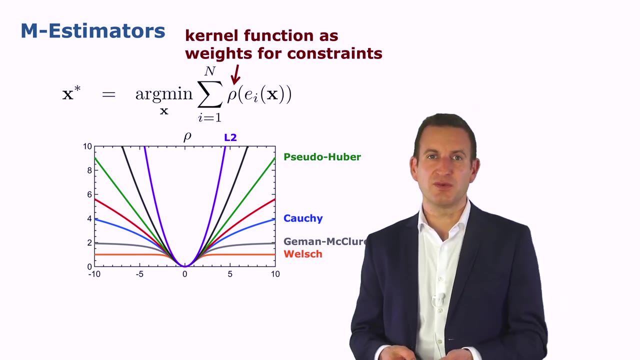 Basically if we are adding wrong loop- closure constraints, for example- And so the key idea in here is to not rely completely on the least squares formulation, but modify the least squares formulation a bit in order to be able to be less sensitive with respect to mistakes that we are doing. 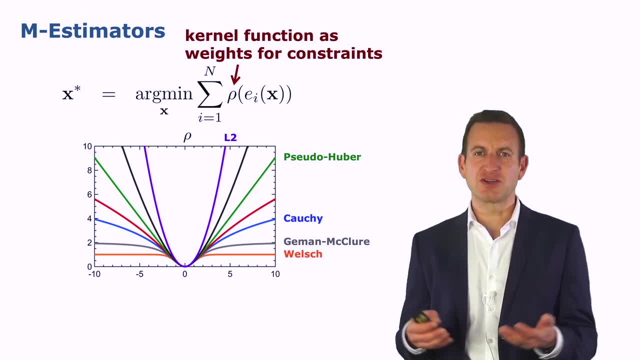 And the key idea is to change the squared error function that Giorgio was introducing in the previous video and replace this squared term by a so-called robust kernel. It is basically a function which changes the shape from a quadratic function to a differently shaped function. 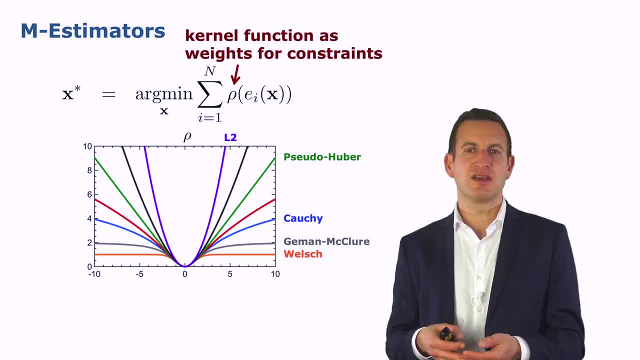 So you can see here on that plot, differently colored functions, And the purple one is actually the robust function, the parabola, the standard, least squares solution. And if we choose a differently shaped function, such as the Cauchy function shown in blue over here, 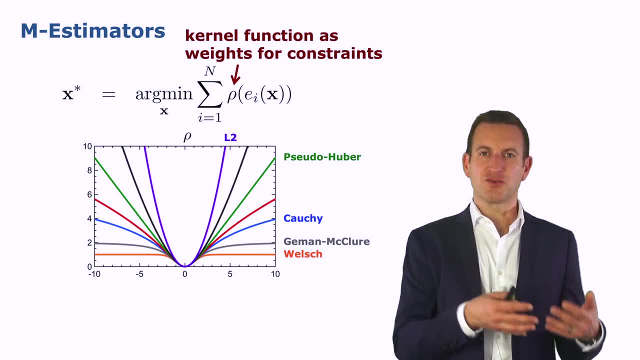 or the Huber shown in green, we can see that the effect of constraints which have a large error- that means they are further away from zero on the x-axis- is lower compared to the quadratic error function, And the key idea is that we can basically choose one of those robust kernels. 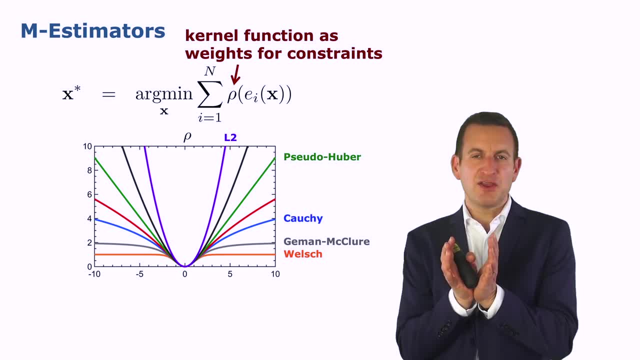 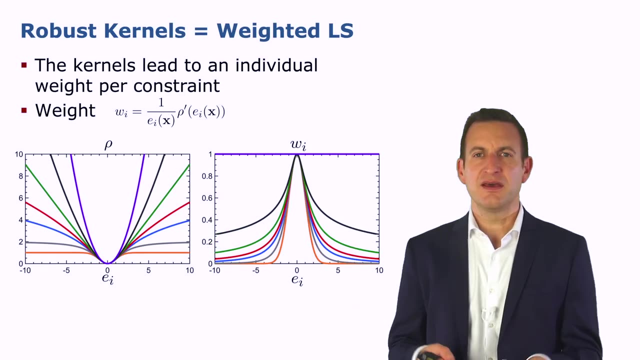 and if we are close to zero error configuration, we basically have a least squares problem. and if we are far away, we are in a problem where the effect of those bad constraints or wrong constraints is substantially downweighted. And the key insight in here is that these robust kernels- 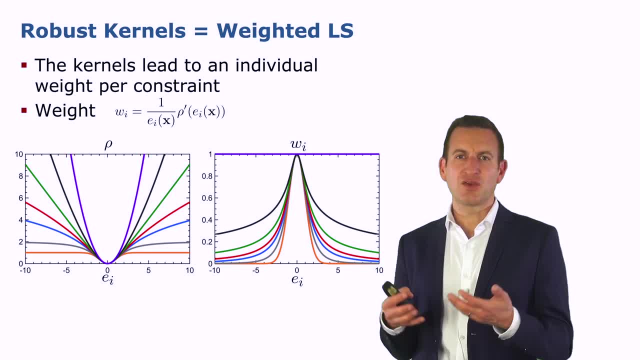 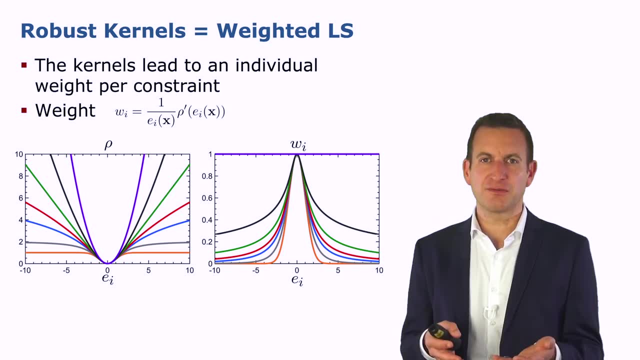 can be used as a weighted least squares problem. That means we don't need to change the math behind it. We can use a different function than the squared error function. So what we need to do? we need to add an additional weight to the minimization term. 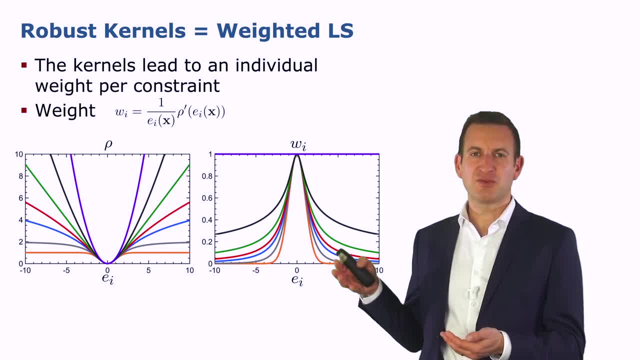 So if we commit on one kernel, let's say the Huber kernel here shown in green, then we have to pick a specific weight shown on the right hand side in this graph, and select the weight value and downweight that constraint if it has a large error configuration. 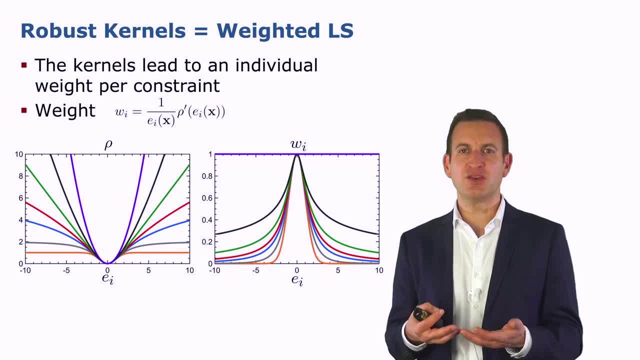 So the purple horizontal line at one means the weight equals to one. in this case we are in the standard least square setting and we don't need to add an additional weight on a different kernel. then we will have to add an additional weight to that, And so we basically select a kernel. 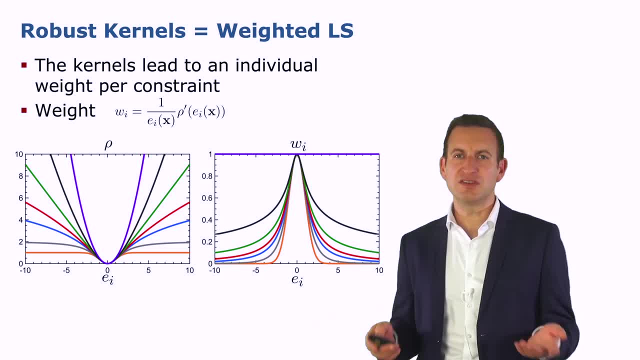 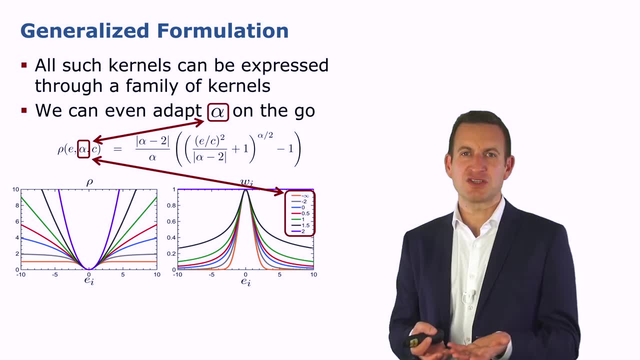 and then perform the optimization with this kernel in order to reduce the effect of outliers in our data cessations. We can even go a step further and use a different type of function, which is basically a family of those kernels shown here in this equation where we have an additional parameter, alpha. 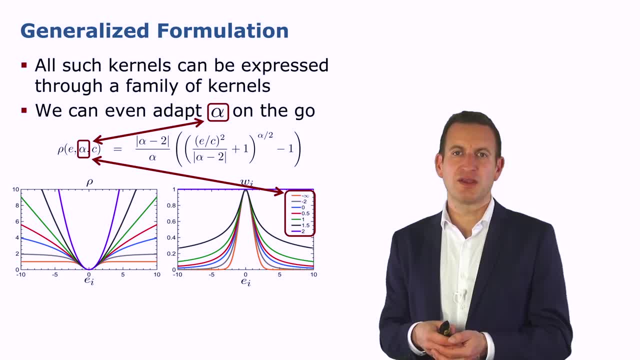 and depending on the value of alpha, we are basically changing the shape of these kernels. So we may take a very low value for alpha and in situations where we are extremely certain about what is going on, we set alpha to two, because then we are in the least squares approach. 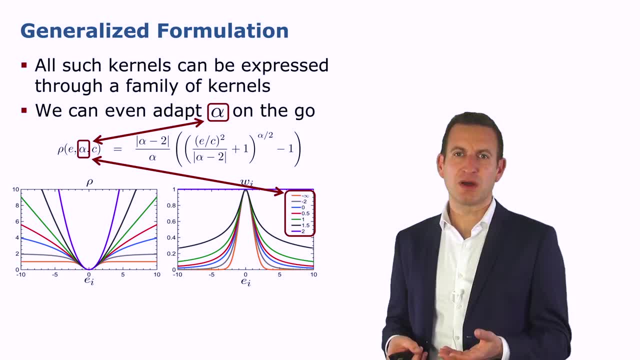 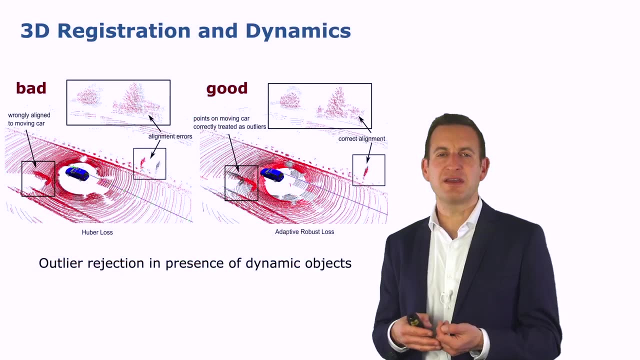 And we can basically turn the optimization problem of finding the best configuration, minimizing the error and, at the same point in time, selecting the correct kernel for our situation. So I brought you an example to illustrate this effect. here you see a vehicle driving over a highway and then it is very likely. 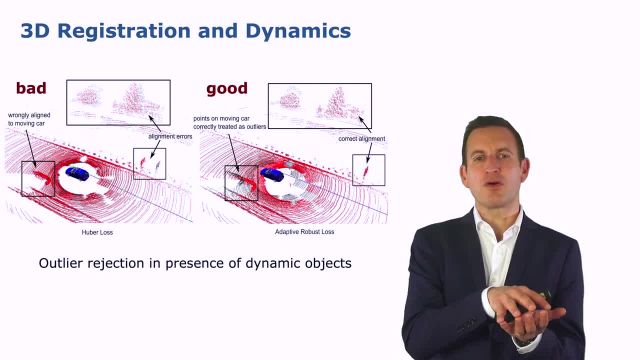 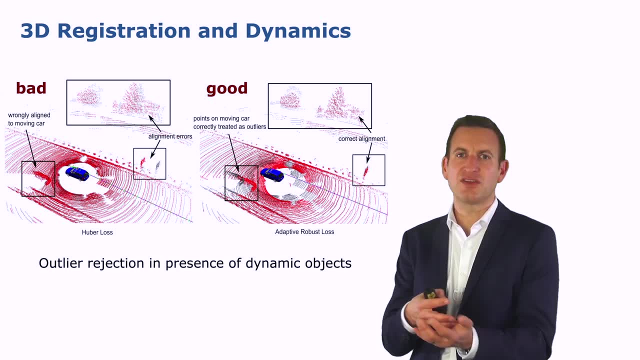 there are not many features around that. the registration system may hook to the wrong car And shown here on the left is actually the result, with the Huber loss where the car committed on the wrong data cessation compared to the adaptive loss on the right hand side. 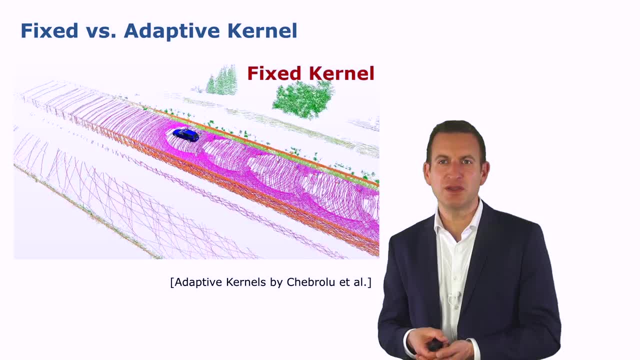 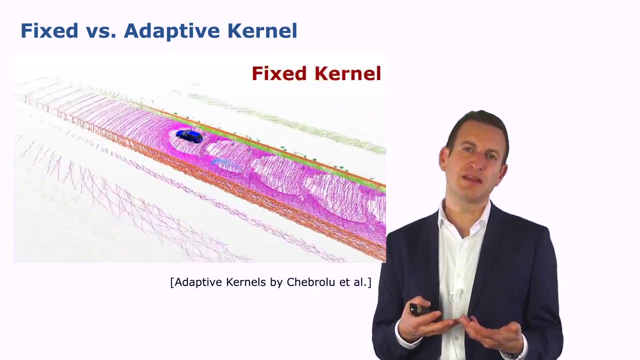 where everything looks good. It may be a bit hard to see from those images and therefore I brought you a video illustrating this. So first we show the result. with a fixed kernel such as Huber, we see the car overtaking and very soon we will make a data cessation mistake. 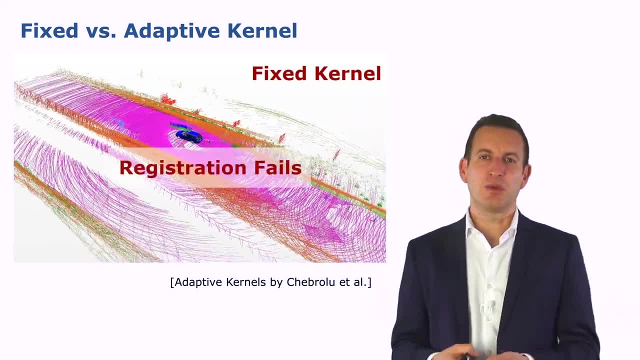 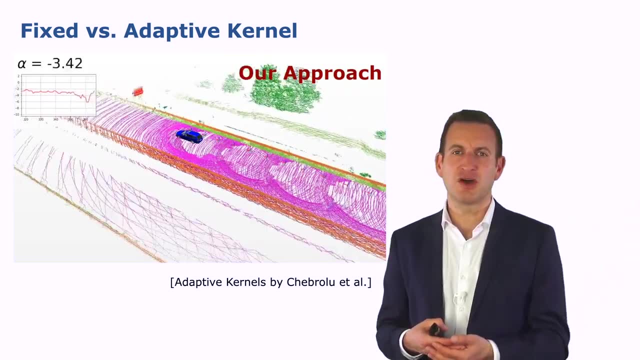 committing to the wrong data cessation hypothesis which we see now and we will end up with a wrong map of the environment If, in contrast to this, we use an adaptive kernel where you see the alpha value here on the top left being adapted to the current situation. 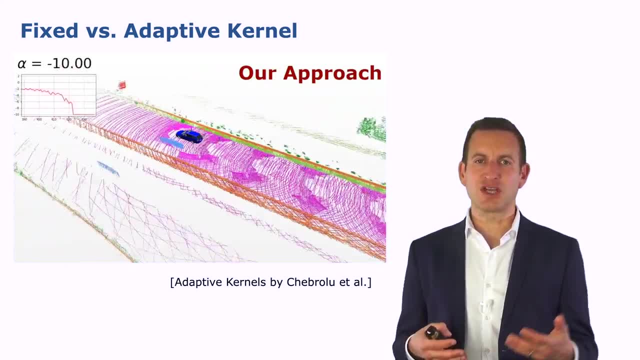 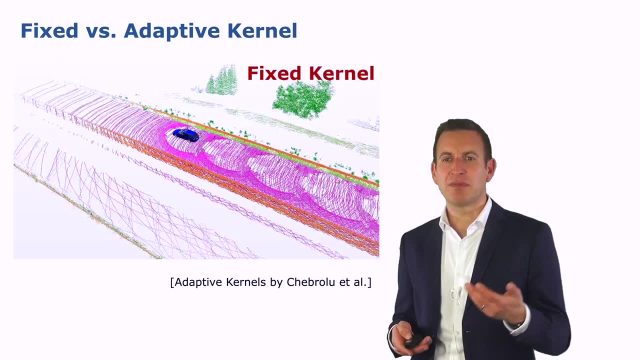 as soon as the car overtakes. we are changing into a mode with a strong outlier rejection technique- here shown with alpha equals to minus 10, but then we are able to build a correct map of the environment. This is the work done by Nived Chabroulu. 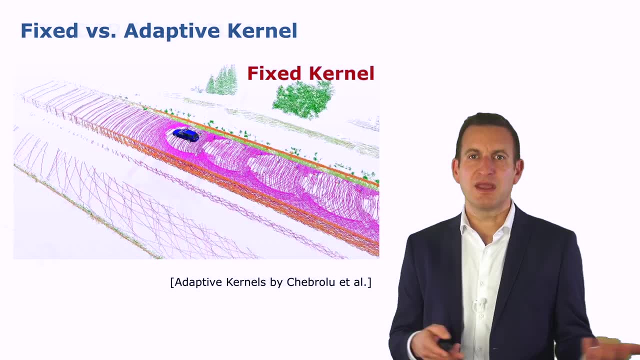 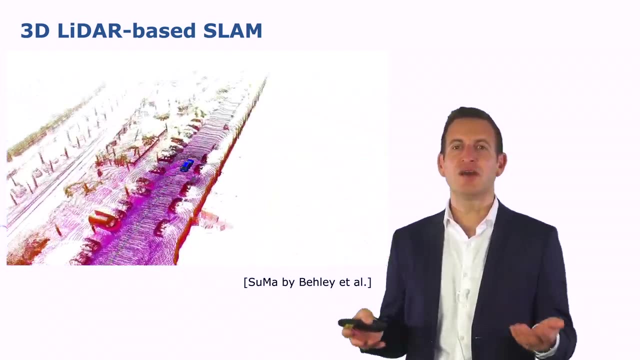 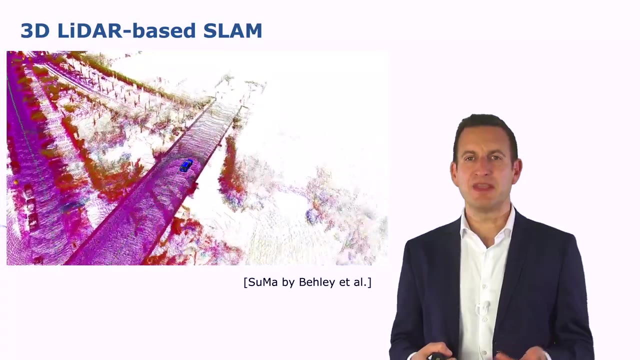 showing how to use those kernels. in the context of this slide problem, We use these ideas- the pose graph, the least square error minimization and those robust kernels- so all the elements shown here within these three lectures- and integrate them into a SLAM system. one example for this is SUMA. 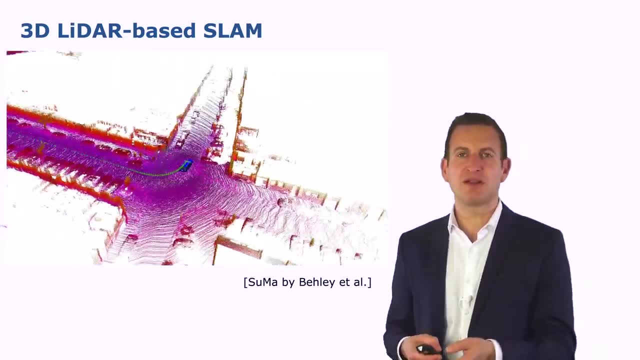 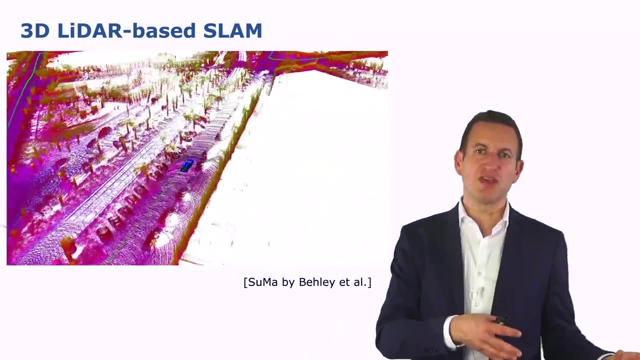 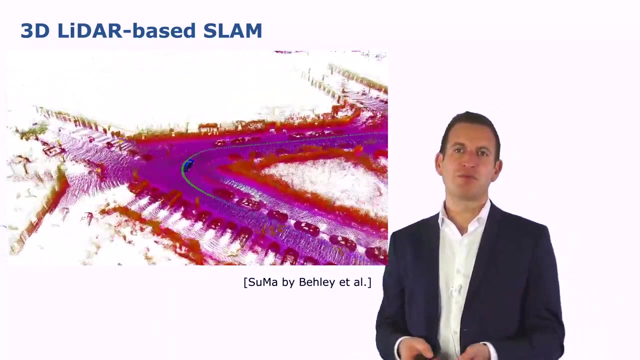 by Jens Belay, which is a LiDAR based SLAM system which is used, for example, in autonomous driving applications. building a map of the environment, building up a pose graph, finding loop closures, registering those different parts of the environment, performing the optimization in order to come up. 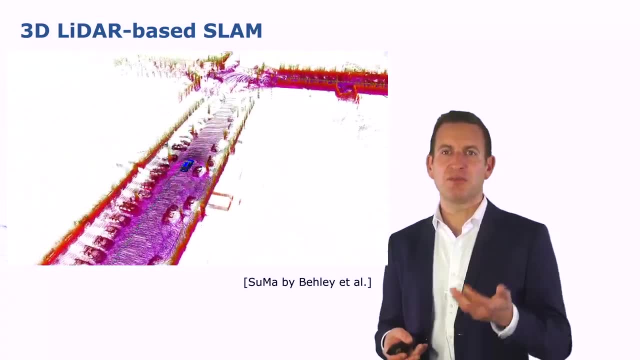 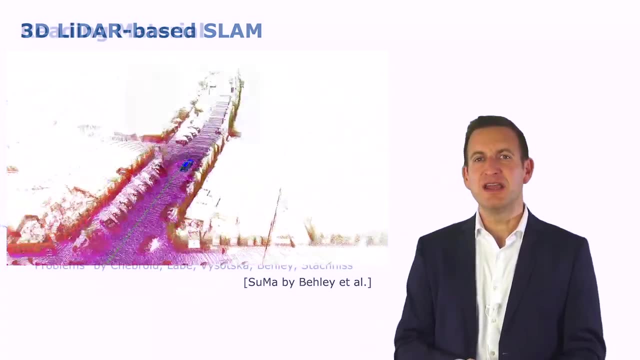 with an appropriate map of the environment, and this is a system that you can build if you integrate the techniques that we have been presenting here into a single system. If you want to dive a bit deeper into SLAM and graph based SLAM, I also brought you some recommendations.